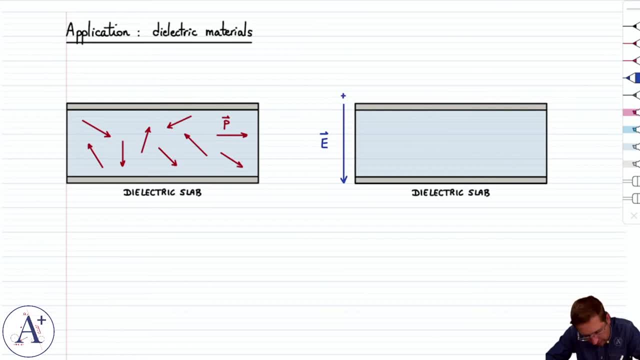 then we know that dipoles rotate in an electric field so as to align their dipole moment with the applied electric field And therefore all these molecules are going to rotate to align their dipole moment P with the external electric field. Now it's worth noting that these molecules cannot flow through the slab. 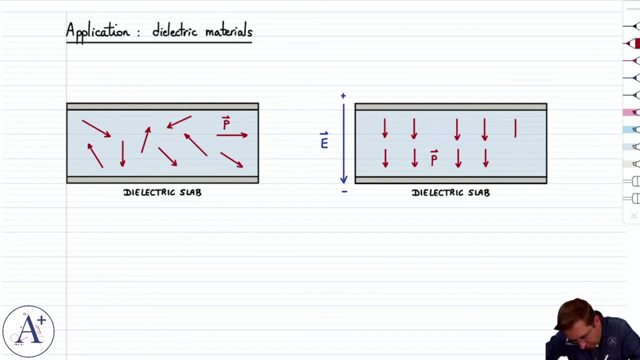 In a sense they're stuck in place, But they are able to rotate and therefore they can align all of these dipole moments with the electric field E. Now the net effect is the following: If you remember, each one of these goes from minus to plus. right The dipole. 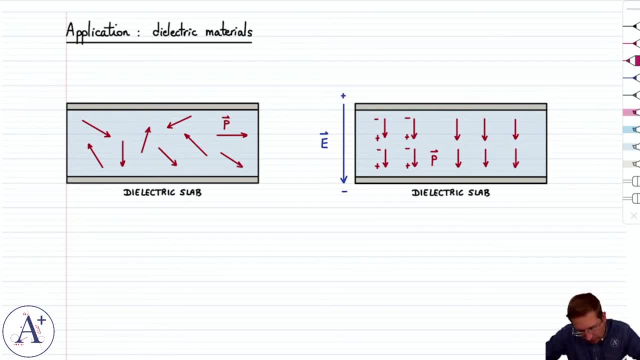 moment goes from minus q to plus q And therefore from plus to minus. everywhere we get a small electric field, E, for each dipole. But if you put them all together you actually find that it's not that small of an electric field And you get what's called E polarized. That's because 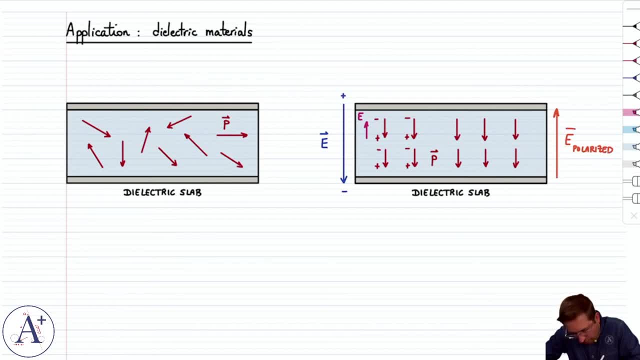 you effectively have polarized your slab. So now your dielectric slab is said to be polarized due to the alignment of all these dipole moments with the electric field E, And because of it the net electric field across the slab is going to be equal to E minus the response from the slab. 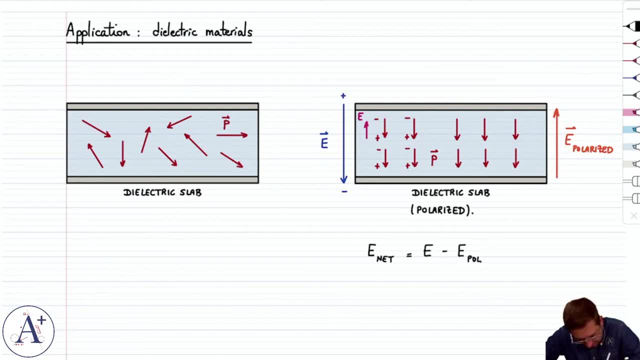 which is E polarized. Now, it's a response, So at best it's going to be equal to E in magnitude, but it can never be greater. So typically you'll find that E is greater than E polarized, And this 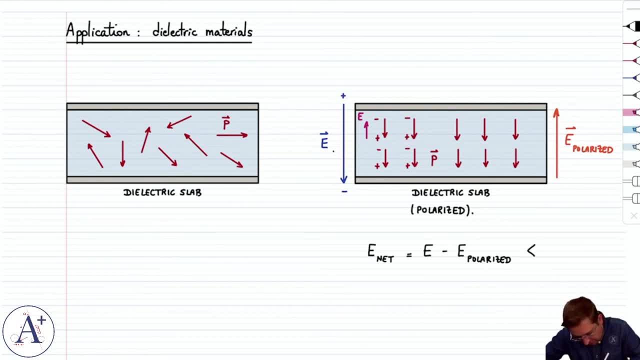 quantity is positive But, more important than being positive, it is less than what you would get if you had a dipole moment. So if you had a dipole moment, you would have a dipole moment. You only had the electric field E, In a sense, these dipoles aligning the way they do. 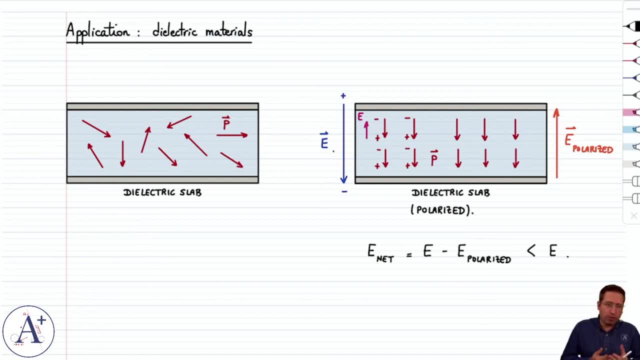 dampen the effect of the electric field by polarizing your slab. Now, this is going to be very important when it comes to capacitors, and we'll talk about it more there, But for now, what we want to do is first acknowledge this and, in a sense, explain why dielectric materials are. 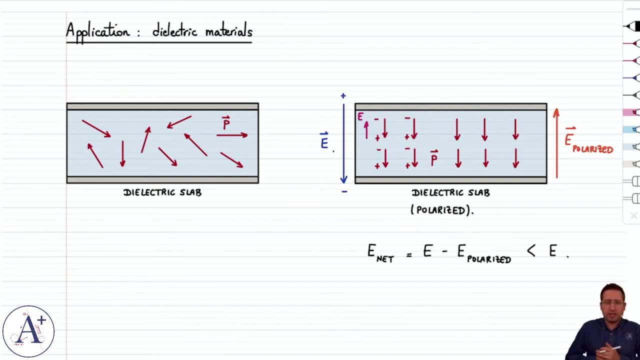 insulating materials. It's because of the polarized electric field that you get E polarized, that dampens the electric field that initially you apply across the slab And we want to characterize the strength of our dielectric. So to do that we're going to 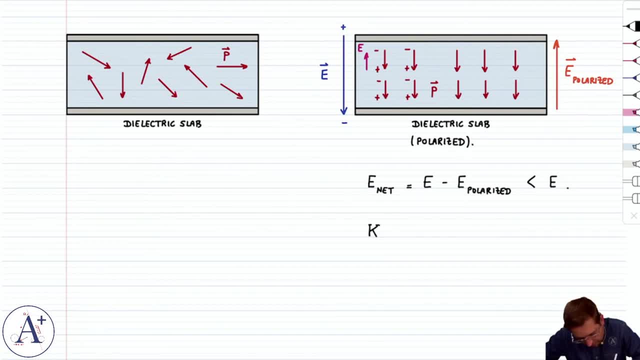 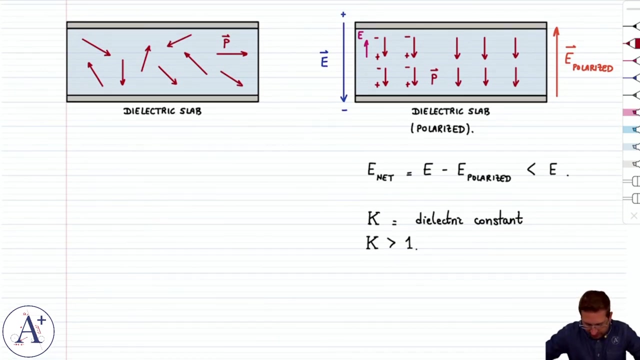 introduce kappa, which is the dielectric constant. And kappa is an interesting quantity because kappa is strictly greater than 1, and a given dielectric has a given value of kappa. But the way that kappa comes into play is that we're going to define a permittivity epsilon for the dielectric epsilon sub d. 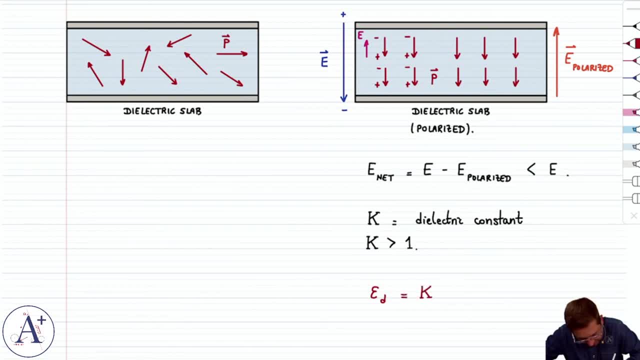 and that's going to be kappa times. E, E, epsilon 0, the permittivity of free space, And, if you remember, epsilon 0 measures how easily you can establish electric field lines in a vacuum, or you can think of it as that, for simplicity anyway, And so the vacuum ends up being 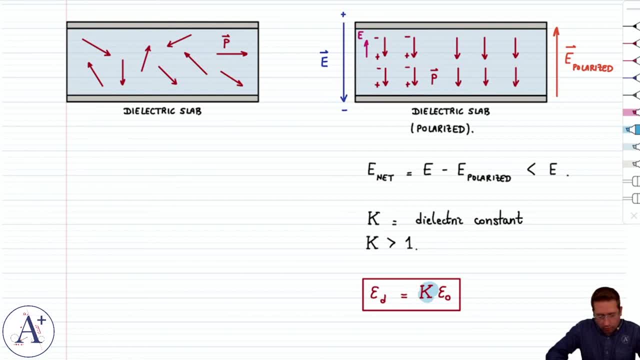 your reference, and because kappa is always greater than 1,, strictly, epsilon d is always greater than epsilon 0. In other words, because kappa is strictly greater than 1, you have a material, a dielectric, that does a better job at insulating than just vacuum. 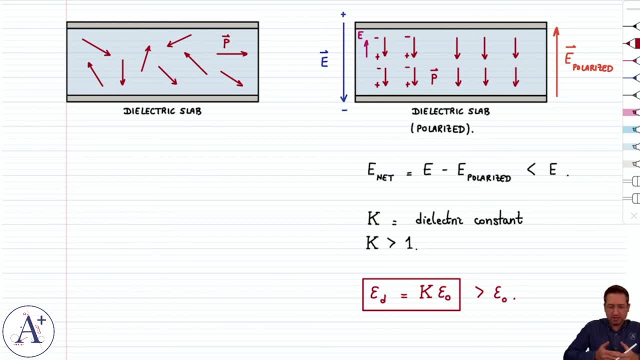 And again this ties back to capacitors. This is why you might place a dielectric slab between capacitor plates to increase the insulating power, if you will, of the capacitor. What that allows you to have is more charge build up on the plates without any risk of frying your capacitor or with lesser risk.